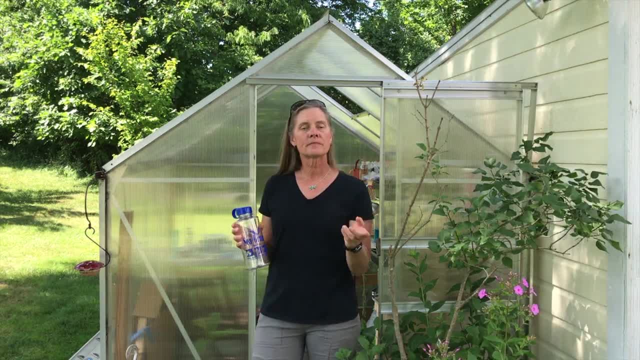 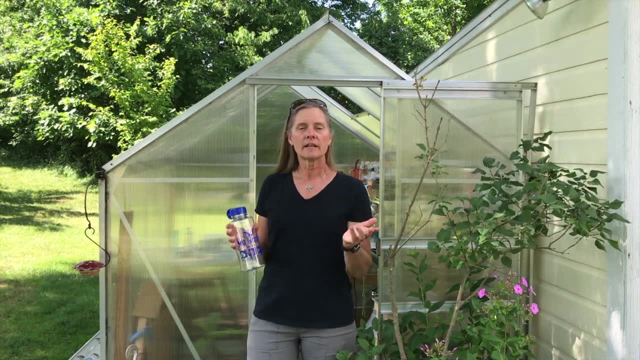 it strikes these gases, they vibrate, and that keeps our atmosphere warm. Sometimes people wonder if these trace gases are actually abundant enough to have any effect at all on the climate. If a molecule like carbon dioxide is just a trace gas, what are the? 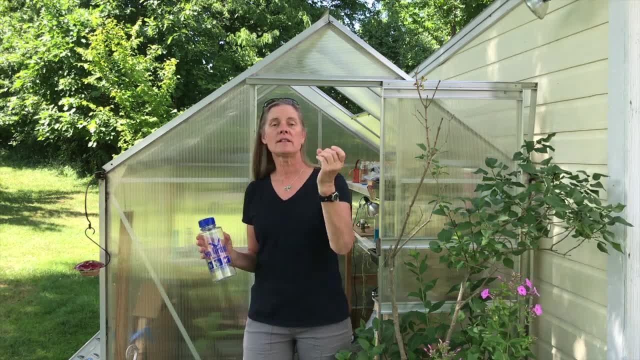 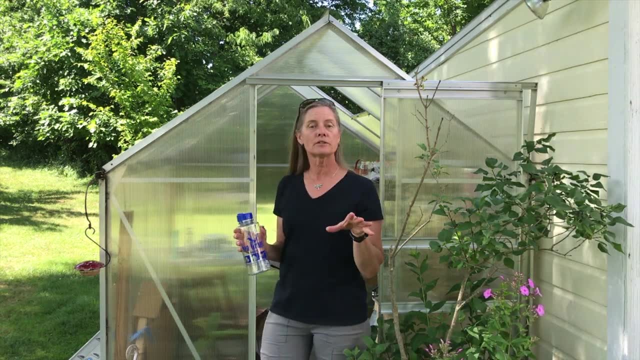 chances that an infrared photon would even strike a CO2 molecule and make it vibrate. Well, why don't we calculate how many CO2 molecules are present in a much smaller volume of air? How about a one liter bottle? And even though that might sound like a complicated 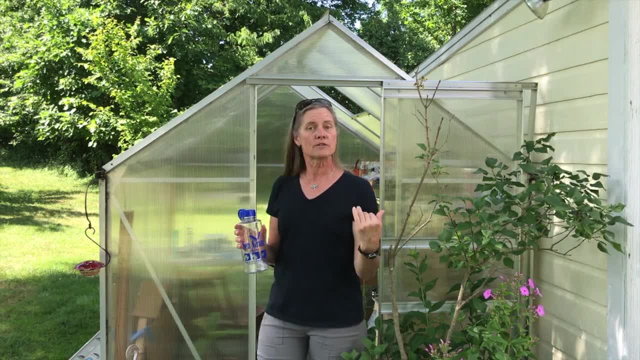 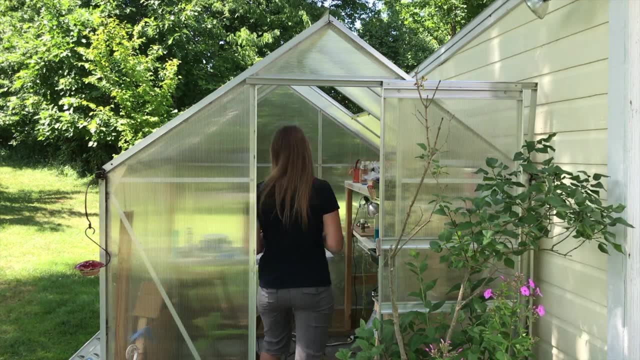 calculation. I can actually do a quick and simple version in my head, But you know what, Since this is a video, I'm going to write it down for you, So come on. Most of the atmosphere is composed of nitrogen and oxygen. These two gases are transparent. 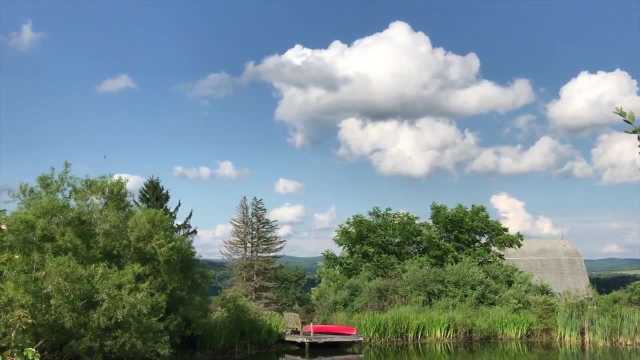 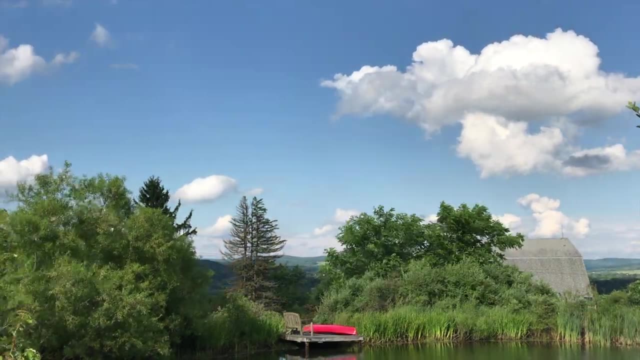 to visible sunlight and infrared energy. Other gases that are important in Earth's climate system are much less abundant. They're trace gases, a gas with an abundance of less than one percent of the atmosphere. Some of the most important trace gases, like carbon dioxide. 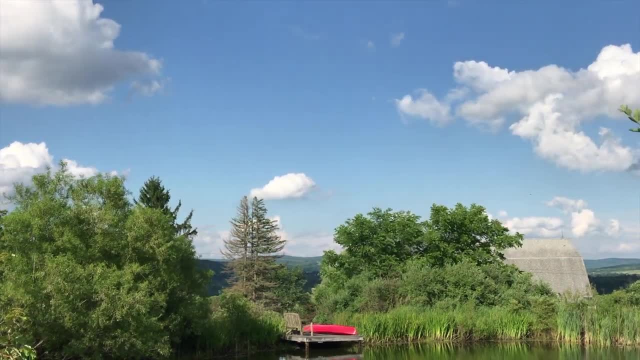 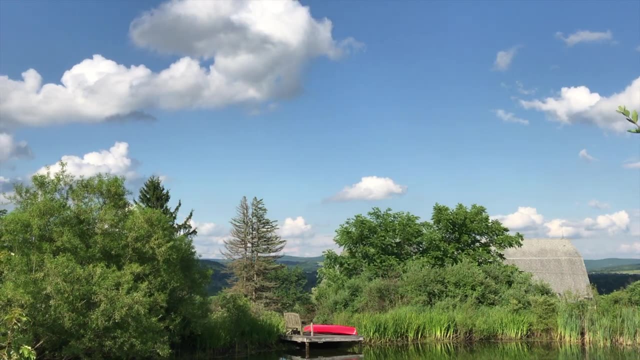 and methane also happen to be greenhouse gases, gases that absorb infrared energy at the same time, that are emitted by the Earth. Carbon dioxide's abundance right now is 415 parts per million. That is, for every million molecules of air, 415 of those are CO2.. CO2. 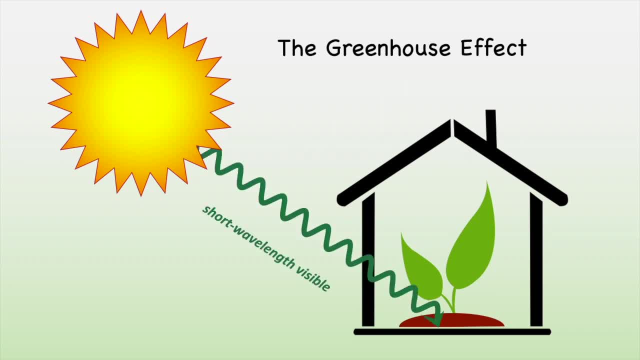 is called a greenhouse gas because it's transparent to incoming visible light, just like the glass in a greenhouse. But just like glass it also absorbs the outgoing infrared energy. When molecules absorb energy, they vibrate and cause motion that warms the atmosphere. But 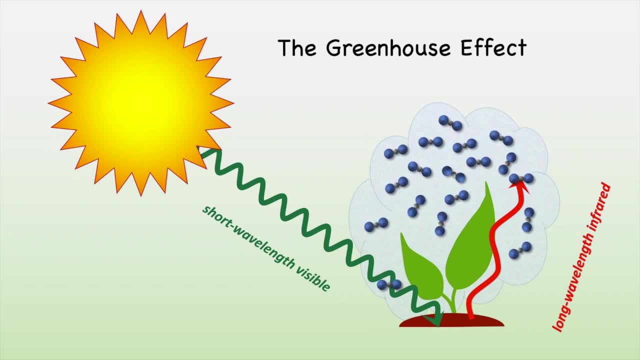 if there are only 415 CO2 molecules in a million molecules of air, how likely are these molecules to absorb energy? How likely is it that an outgoing photon of energy would even hit a CO2 molecule? Instead of trying to think about the whole atmosphere, let's work with 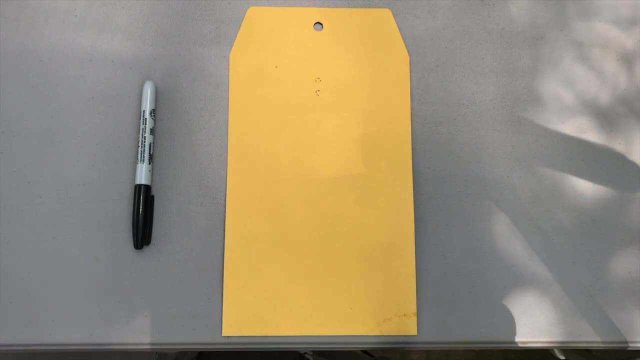 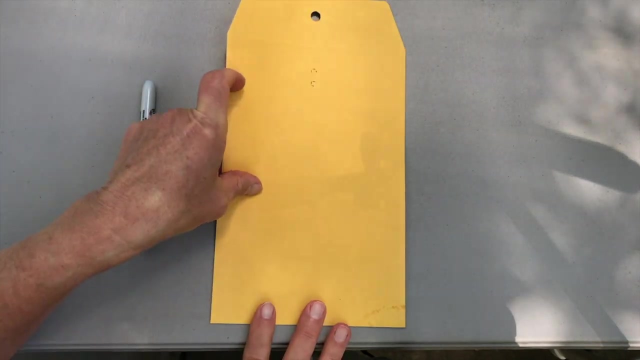 a more manageable volume, a one-liter bottle. I'm going to do what's called a back-of-the-envelope calculation and I'm actually going to do it on the back of an envelope. When we're working with gases, we need to work in units of moles. A mole is 6.022 times 10 to the. 23 molecules. This is called Avogadro's number. To simplify the calculation, I'm going to use 6 times 10 to the 23 molecules. What's the volume of a mole of gas At standard temperature and pressure? 0 Celsius?